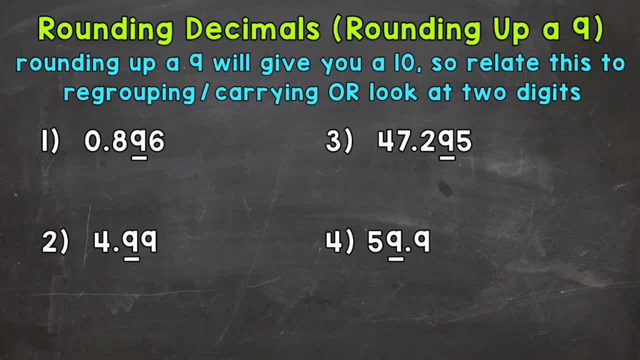 hundredths place is underlined that nine. So let's look to the right and see if we round up or stay the same. So we look to the right and we have a six, Remember five or more, and we round up. So six is five or more, we're going to round up. If we round up a nine, we get 10.. So we put. 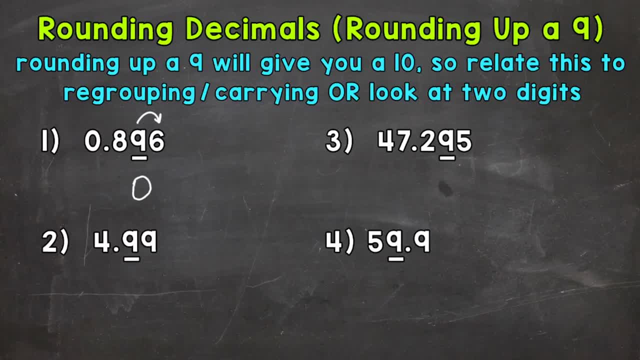 the zero in and we round up a nine. So we round up a nine and we get 10.. So we put the zero in the hundredths place and then regroup or carry the one from that 10 over to the next place to the left, in this case the. 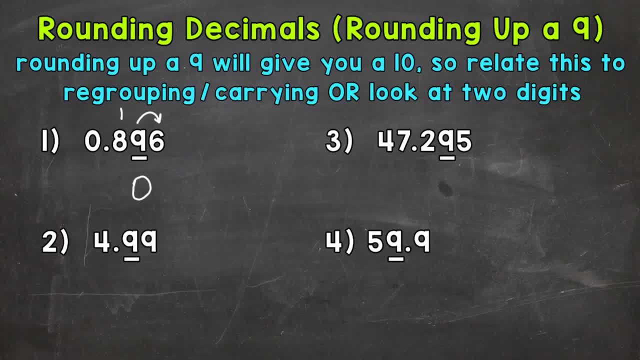 tenths place. So in the tenths we have one plus eight, which is going to give us nine. So 896 thousandths rounds to 90 hundredths. Another way we can think through this. let me rewrite our decimal here. Going to round to the hundredths is: take a look at two. 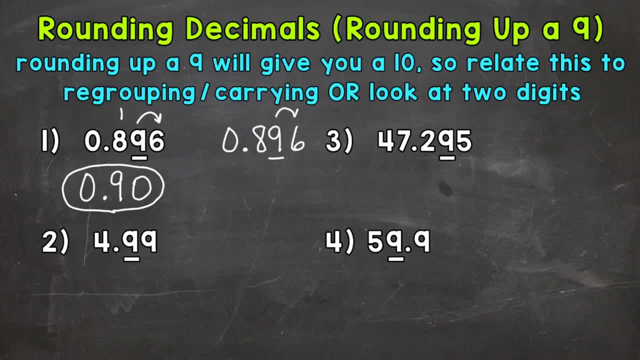 digits. So we're going to look to the right. we know we're going to round up. Let's look at these two digits here: the 89. Think of this like an 89. So we round up an 89. If we round up 89, that gives us 90. So let's put our 90. So we round up an 89. If we round up 89, that gives us 90. So let's put our 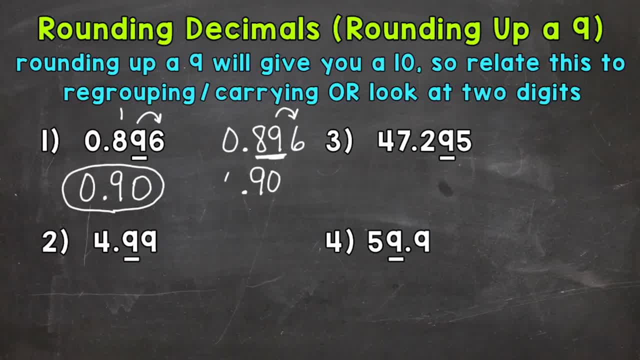 90 here. Put our decimal in and our zero to show that we don't have any whole numbers And we get 90 hundredths that way as well. Let's try a few more examples and move on to number two, where we have four and 99 hundredths. So we're going to round to the nearest 10th. We have the digit in the. 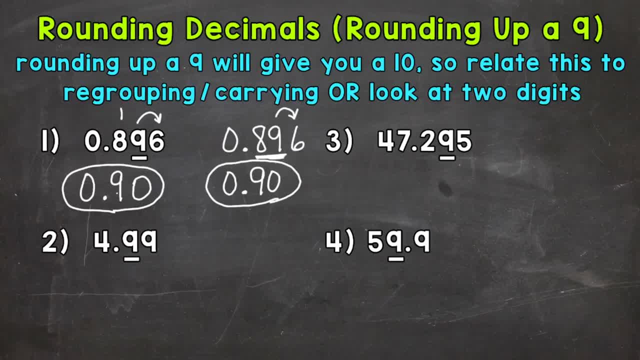 10th place underlined, It's that nine. So look to the right And we have a nine. So we are going to round up a nine. So we round up a nine, So we round up. If we round up a nine, we get 10.. So let's think of this and relate it to regrouping or carrying. So put the zero in the tenths and 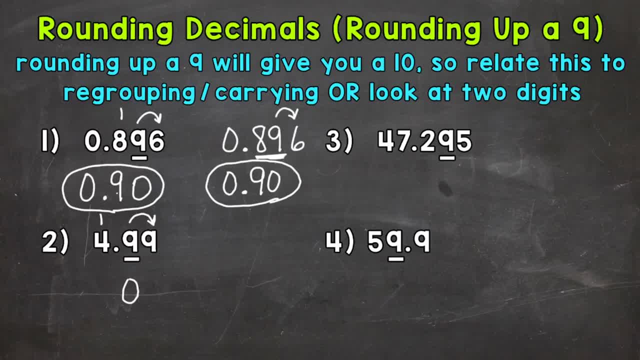 regroup or carry the one. Now we have that one and the four. that's going to give us five. Bring our decimal down in between the ones and tenths place, And four and 99 hundredths rounded to the nearest 10th is four. So we're going to round up a nine. So we're going to round up a nine. So let's think of this and relate it to. 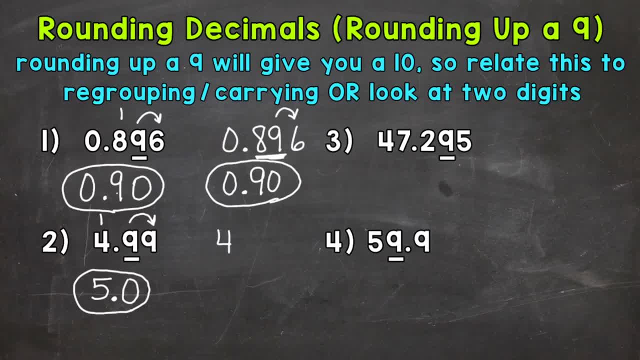 five. Let's try it the other way. So four and 99 hundredths, We're rounding to the nearest 10th. Look to the right, So we round up. Take a look at two digits here, So think of that like 49. If we round up 49, we get 50. But don't forget the decimal in between the ones and tenths place. So we get five that way as well, Let's. 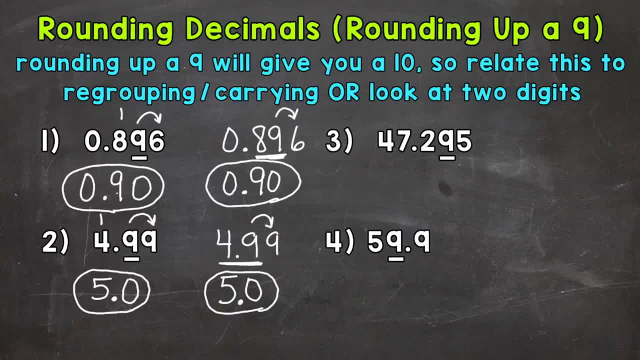 move on to number three, where we have 47 and 295 thousandths. So we're going to round to the nearest hundredth. We have the digit in the hundredths place underlined: It's a nine. Let's look to the right And we have a five, Five or more. we round up. So we're going to round up. Now. if we round up a nine, we get 10.. So let's put our zero in the hundredths and then regroup or carry the one. 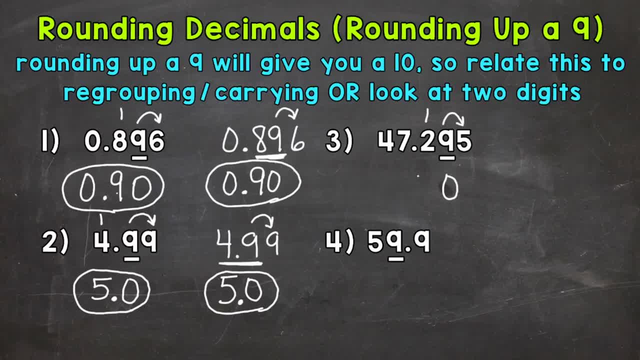 One plus two gives us three in the tenths place. Put our decimal in and then the whole number. So 47 and 295 thousandths rounds to 47 and 30 hundredths. when we round to the nearest hundredth, Let's try the other way as well. So nearest hundredth. 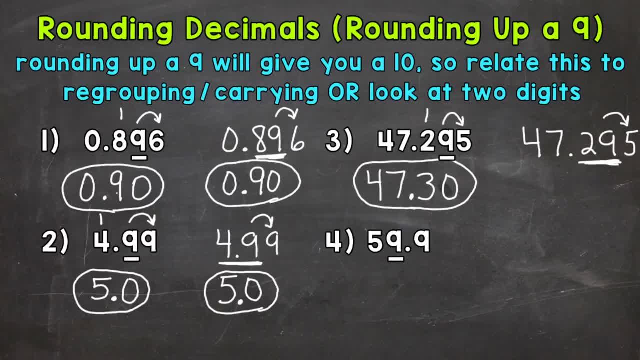 We know we're rounding up. So look at these two digits here: 29 rounded up is going to give us 30 hundredths, Include our decimal and whole number, And we get the same thing that way as well. Lastly, number four: we have 59 and nine tenths. So we're going to round to the ones place here, also known as rounding to the nearest whole number. The digit in the ones place is: